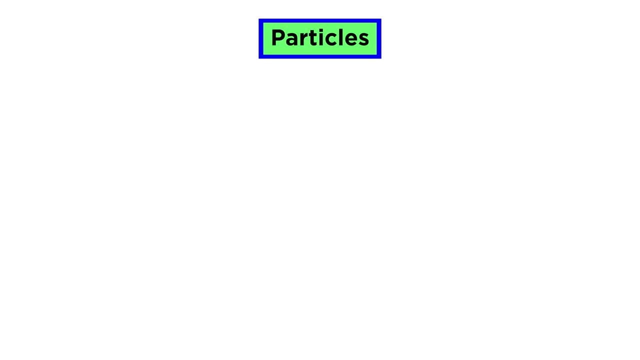 All of the particles in the universe can be divided into two categories: fermions and bosons. Fermions are particles that make up matter and bosons are particles that mediate to matter. Within the family of fermions, there are two types of particles: quarks and leptons. 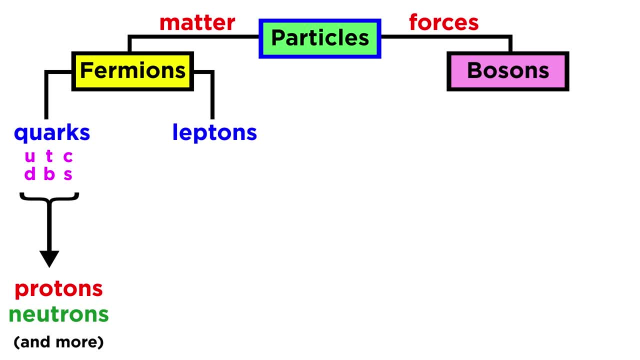 Quarks make up the subatomic particles we are familiar with, the protons and neutrons found in every atom in the universe, and leptons are other massive particles that are not made of quarks, like electrons. On the other hand, in looking at quantum field theories, 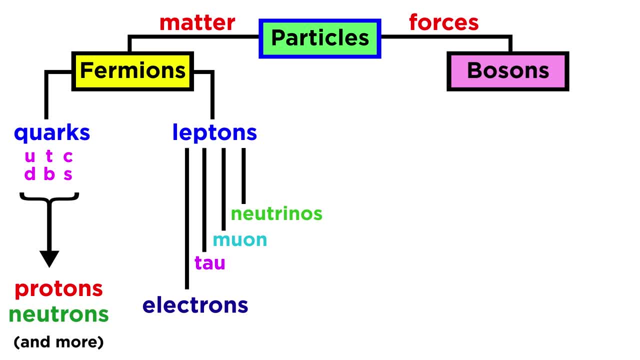 we became familiar with particles that mediate force, which we call bosons. These include the photons that mediate the electromagnetic force, the W and Z bosons that mediate the weak nuclear force, the gluons that mediate the strong nuclear force and the still hypothetical graviton, which ought to mediate gravity. 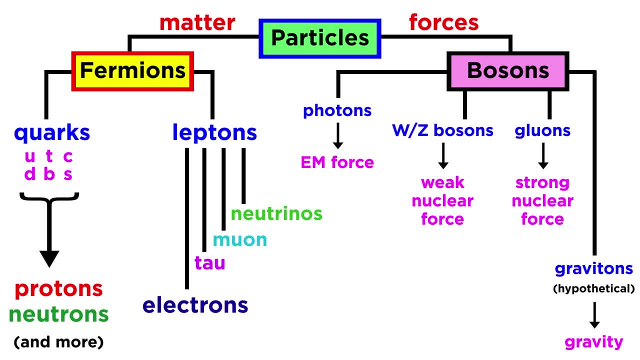 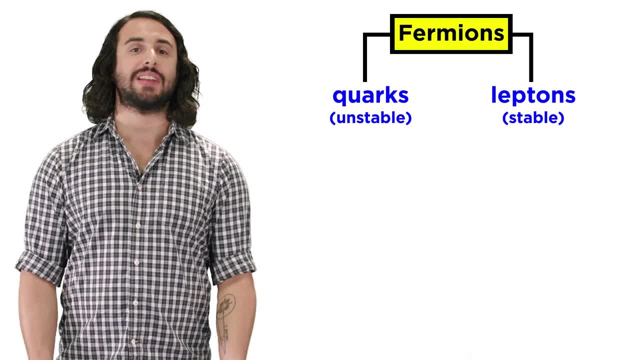 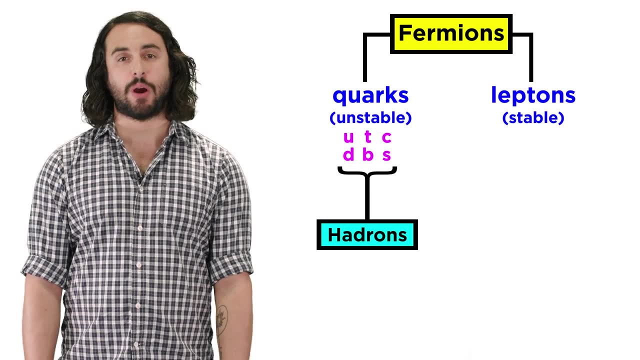 So once again we've got fermions- the particles that don't mediate forces, and bosons, the ones that do. Fermions, as we said, can be split up into quarks and leptons. Leptons are stable by themselves, but quarks are not, so quarks combine to make other particles. 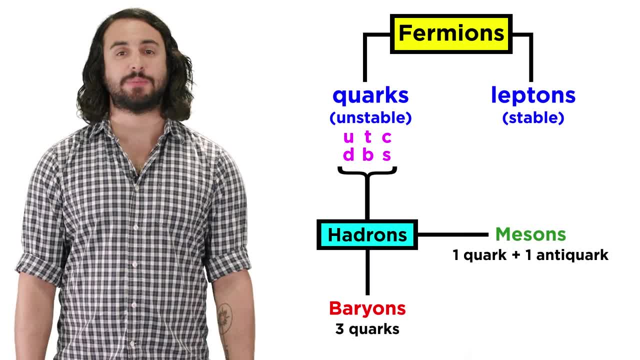 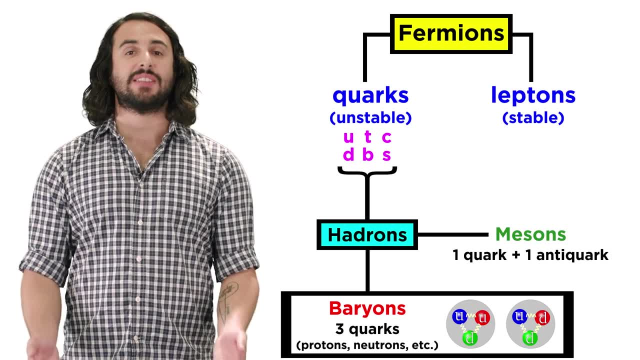 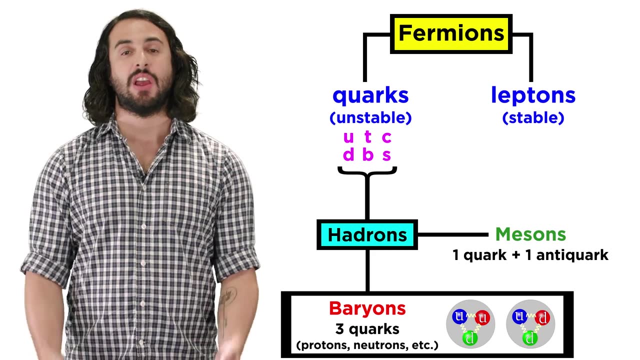 called hadrons. Hadrons themselves can be split up into mesons and baryons, the latter being the nucleons we are familiar with. Protons and neutrons are examples of baryons, but there are many more, given all the possible combinations of three quarks. So far, that leaves us here. We can see. 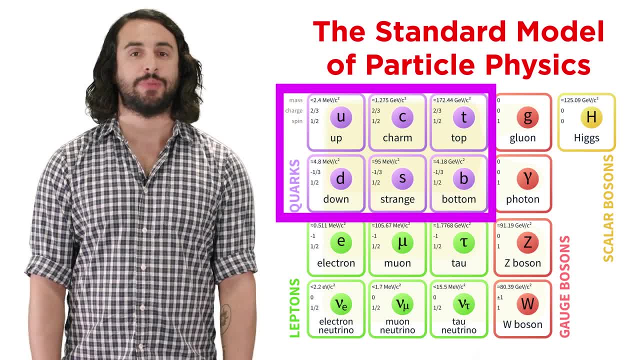 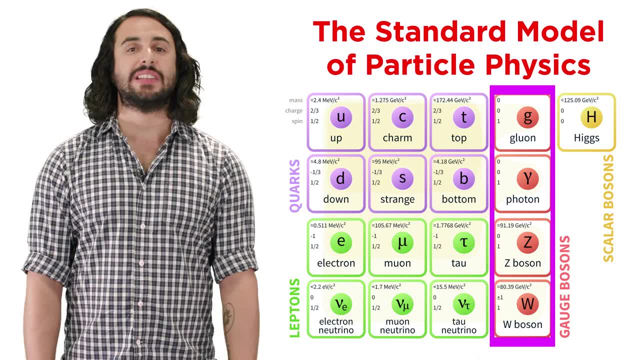 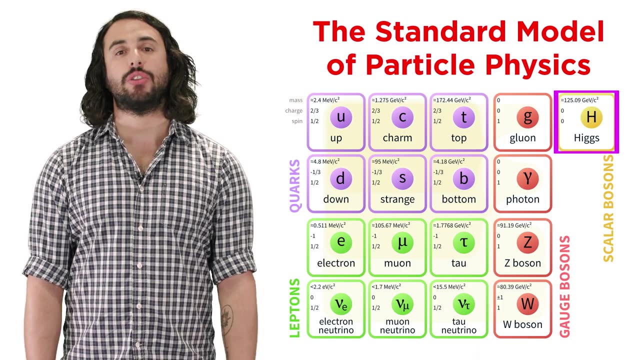 up down, charm, strange top and bottom quarks. We see the leptons, including the electron, muon, tau and their respective neutrinos. We see the gauge bosons that mediate the three forces we have quantum field theories for, and the Higgs boson, the particle that bestows massive particles with. 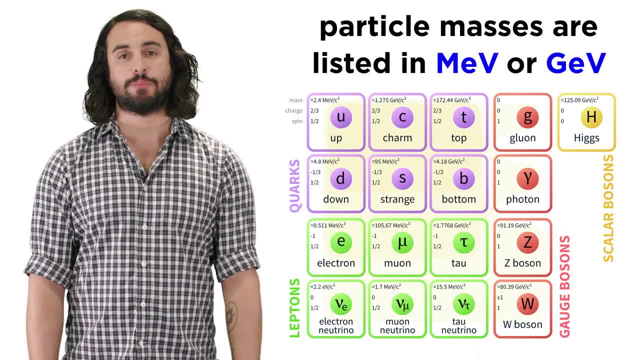 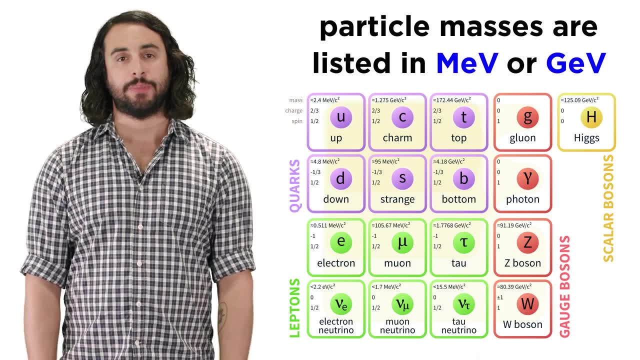 their mass. The rest masses of these particles are often listed in mega-electron volts, a unit of energy, due to mass-energy equivalence. So we can see that the three forces that mediate the force, muon, tau and their respective neutrinos always catch the particles in two parts due to mass-energy. 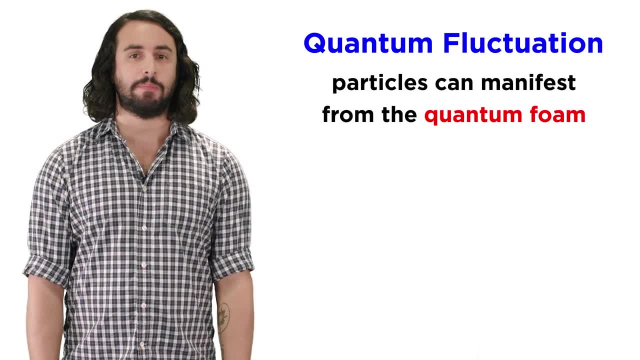 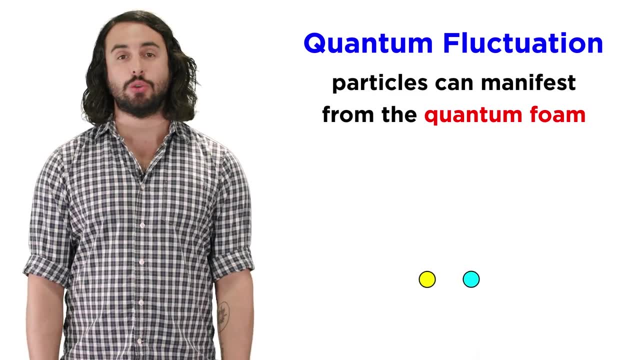 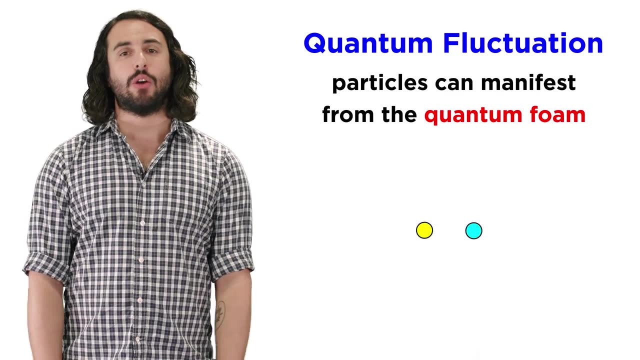 equivalence. But wait, we're not through yet. Remember when we talked about virtual particles that can exist because of the Heisenberg uncertainty principle. These particles appear without cause simply due to their mere probability of existing, but in doing so they always obey. 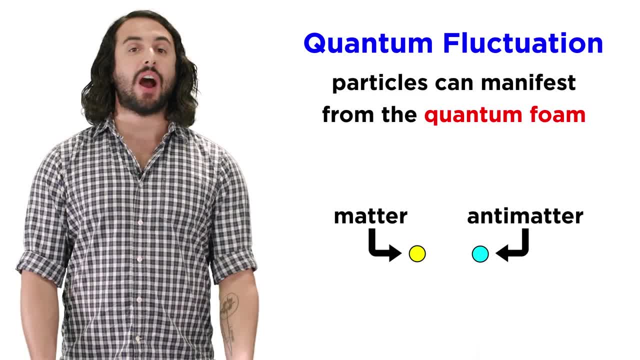 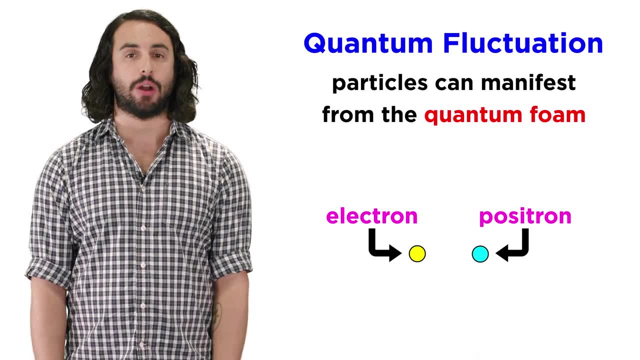 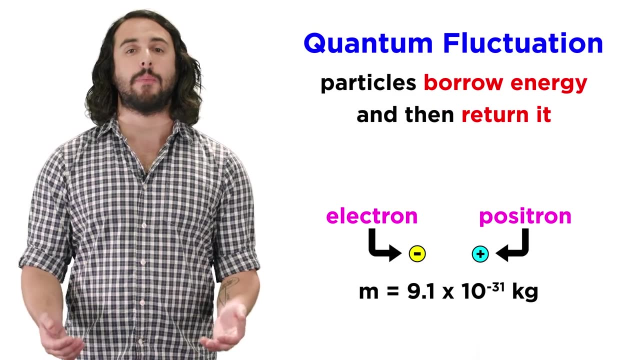 symmetry in that they arrive in pairs. One of these particles is considered regular matter. So when an electron forms, it is not without its antimatter counterpart called the positron. These have the same mass, but they are opposite in charge and just as they are born out of. 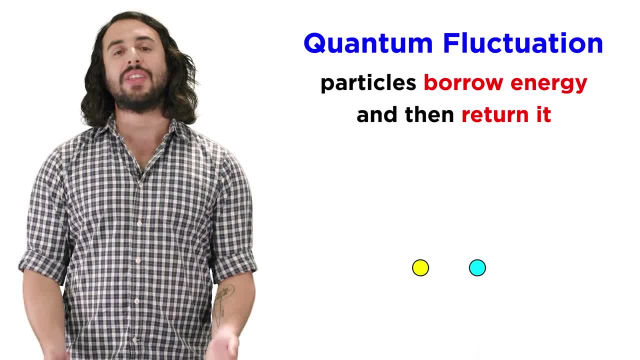 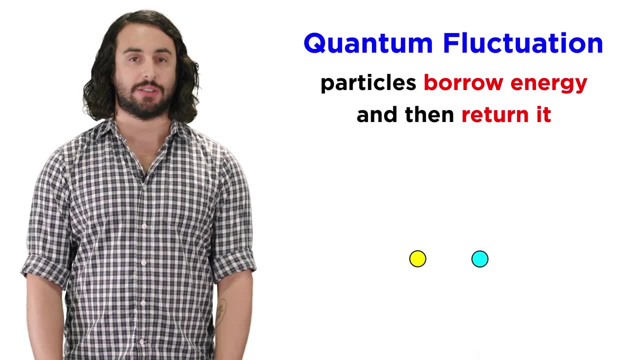 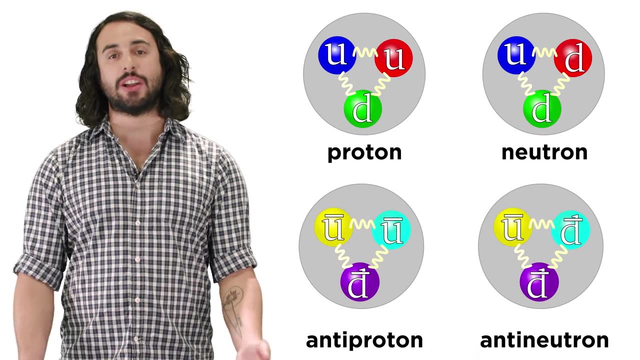 energy, like experiments in particle accelerators: when they collide they annihilate back into pure energy, returning the energy that was borrowed by their existence. Leptons and neutrons have antiprotons and antineutrons that are made of anti-quarks. 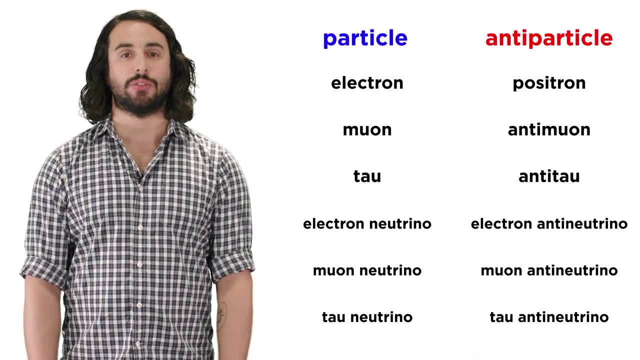 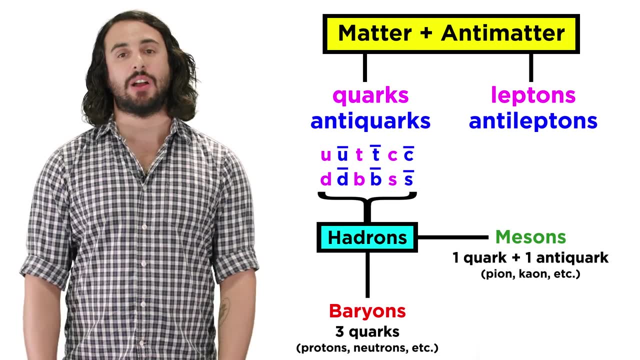 All the leptons have antiparticles too, like antineutrinos. When we include antimatter, the particle zoo gets much bigger, because we can then include mesons, which are short-lived particles comprised of one quark and one anti-quark. 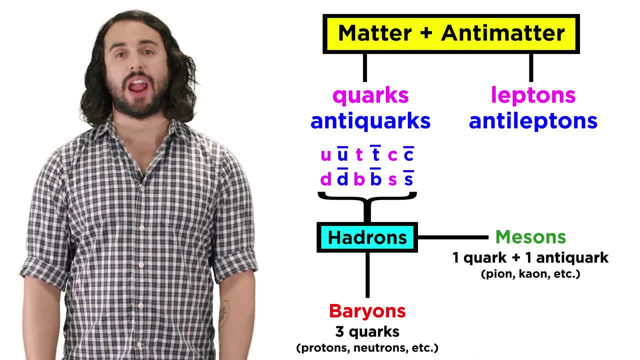 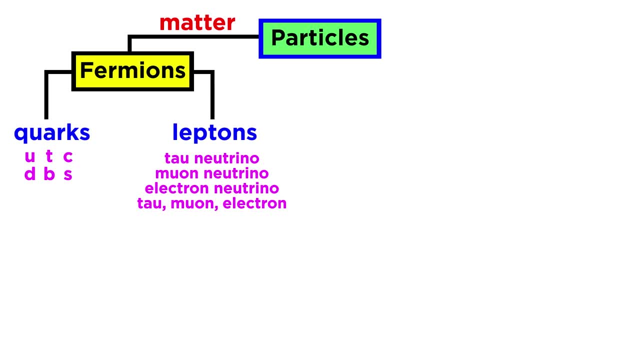 There are plenty more hypothetical particles, but we can pause here and review what we've learned Once again. matter is made of fermions. Fermions are comprised of quarks, which come in six varieties, and leptons, of which there are also six. 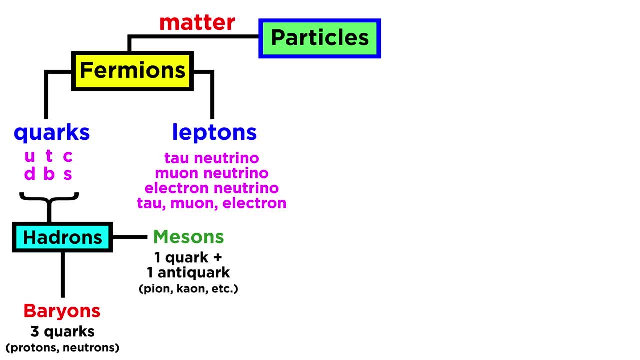 Quarks combine to make hadrons, which are either mesons or baryons, depending on the quark combination. Protons and neutrons are the baryons that make up atomic nuclei, which come together with electrons from the lepton family to form atoms, which then form molecules and all the 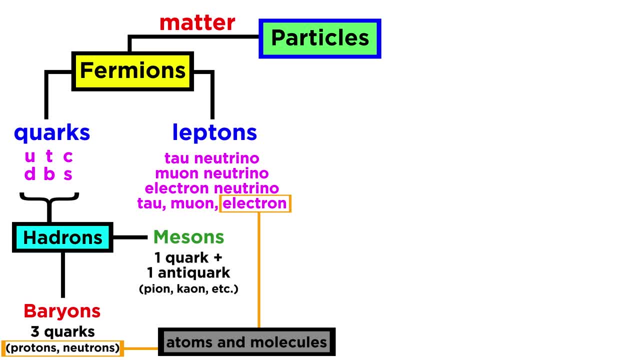 atoms that form the leptons. So let's get started. Let's look at all of the matter we see every day. On the other hand, we also have the force-carrier particles called the bosons. These are the gluons that mediate the strong nuclear force, the W and Z bosons that account.